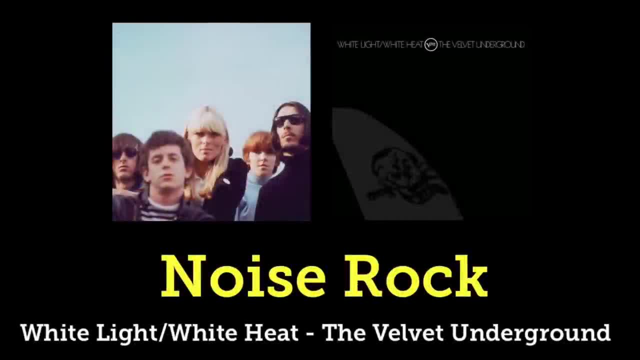 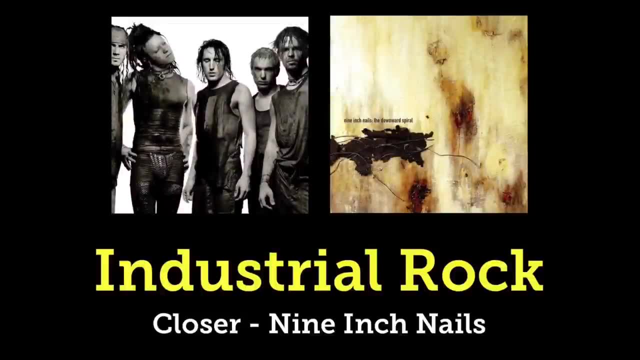 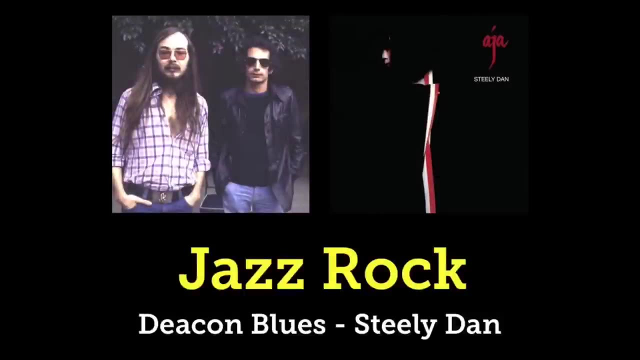 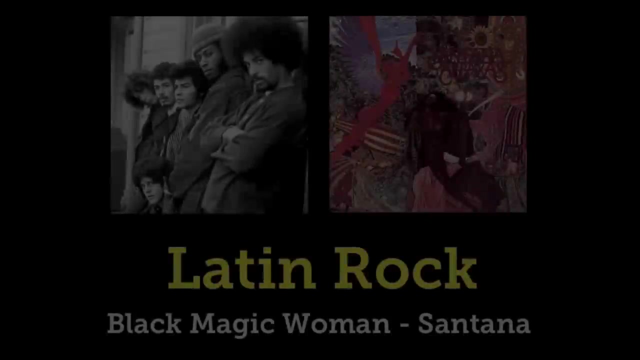 Oh, don't you know I'm gonna make me go blind. Oh why he did to kill me. then My whole existence is flawed. Call me Dejan dejaniu. Turn the wind up. shade off air. I've got a black-minded woman cut me a soap on a knife. 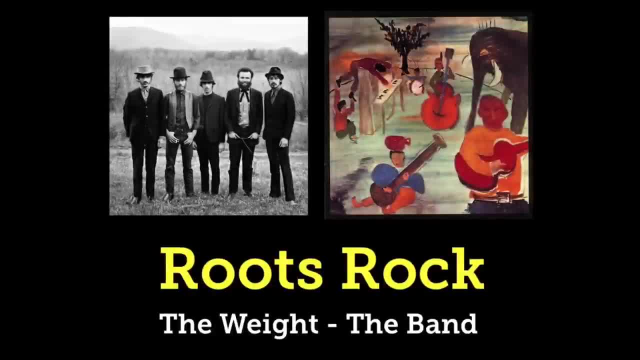 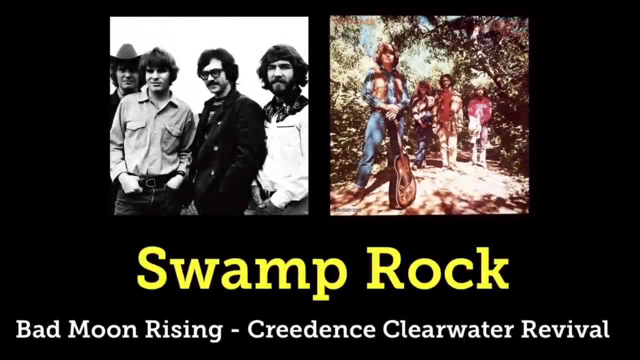 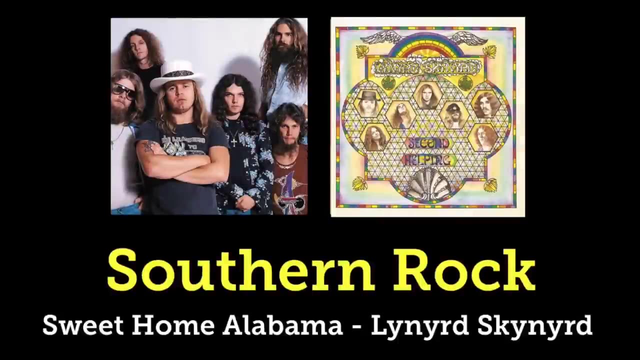 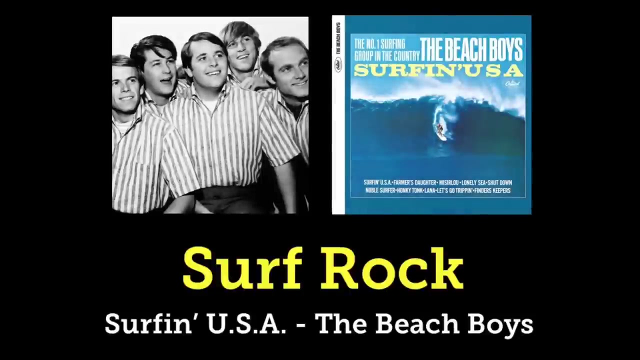 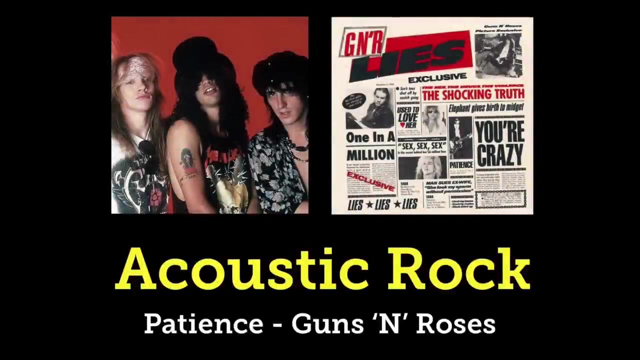 You'll see. You'll see, Take a load off, Fannie, take a load for free. I see the very moon rising. Sweet home, my, my, my, Everybody's got a servant. Servant USA. All we need is just a little patience. 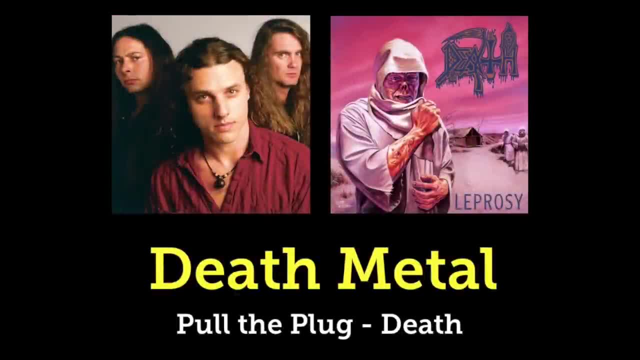 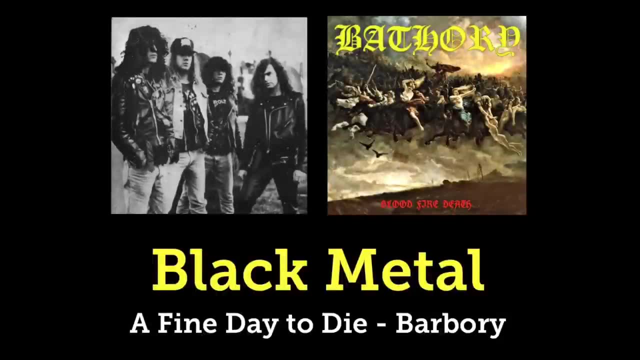 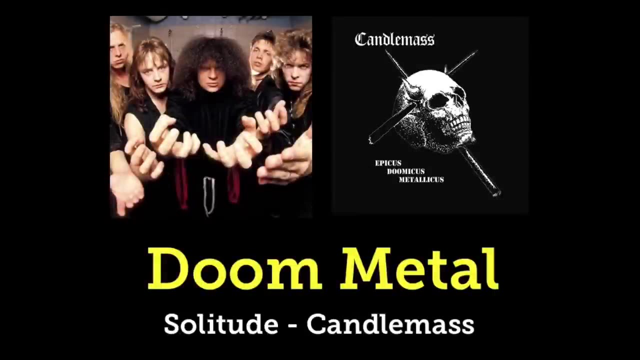 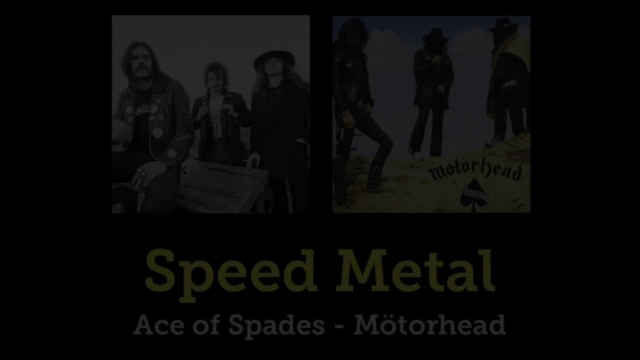 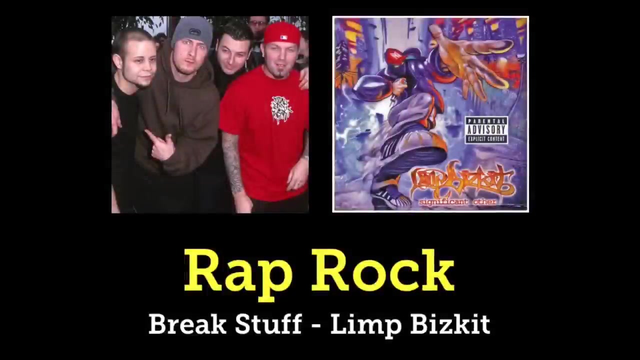 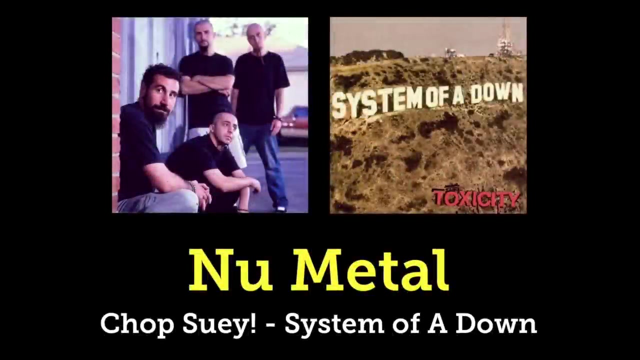 For the one I- I I'm a shade green. The only gun I need is the air. Raise the spades. the ain't Me Spat Walk. I think you better quit, let the shit slip Or you'll be leaving with a fat lip. You wanted to grab a brush and put on a little makeup. 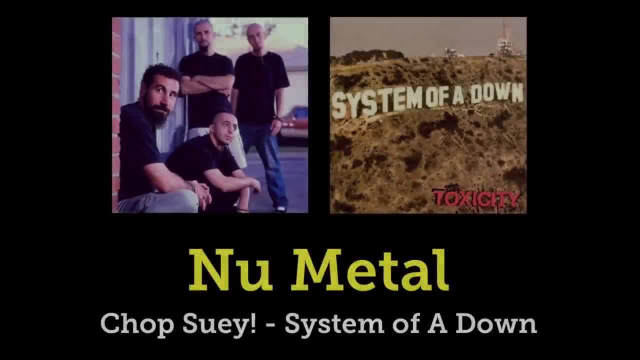 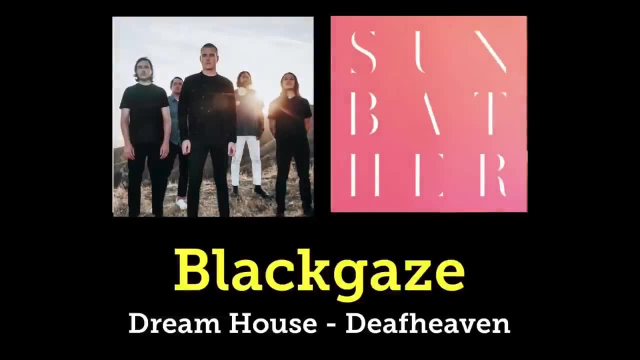 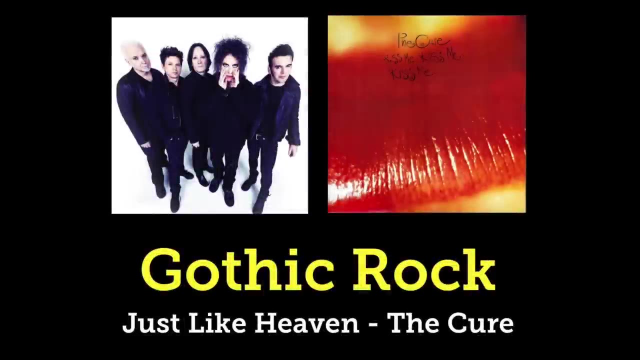 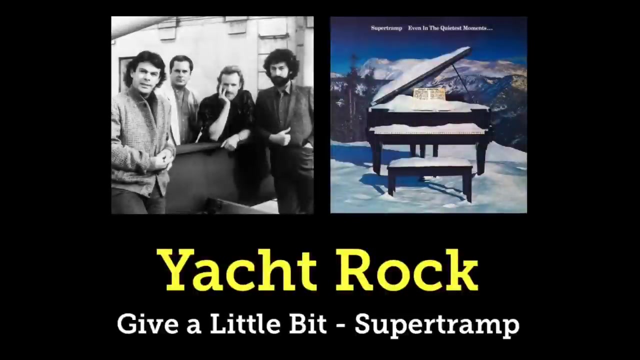 You wanted to. I described the pain and way to shake up. You wanted to. why'd you leave the kids up on the table? You wanted to. why'd you leave us alone? You wanted to. why'd you leave us alone? Walk up the stairs. we're all just strangers. 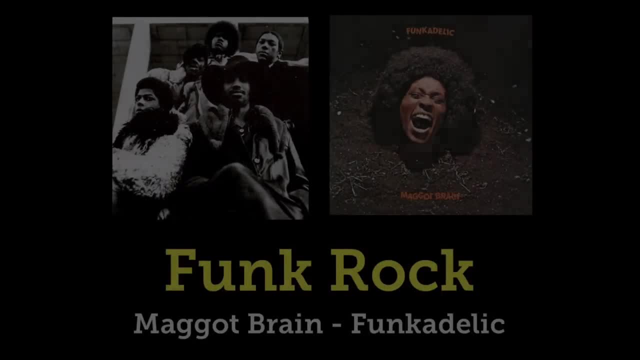 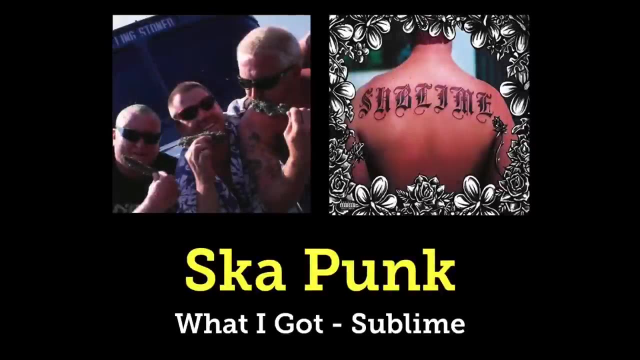